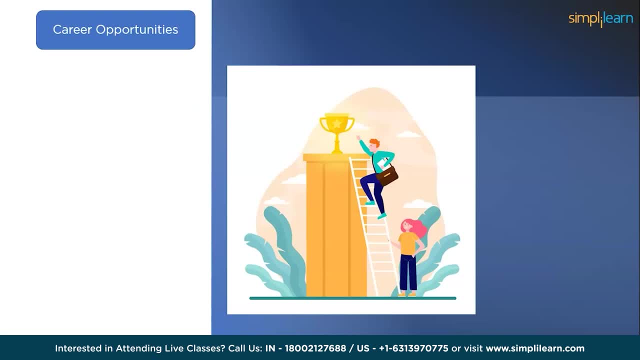 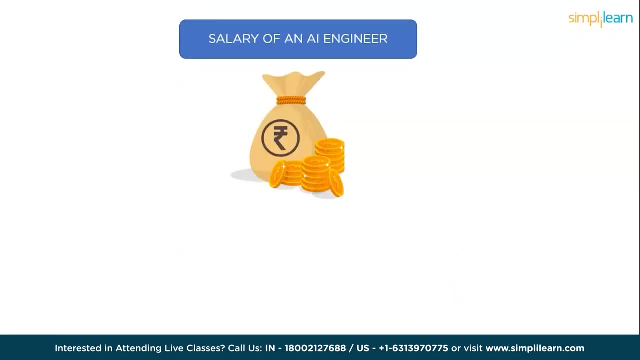 with expertise in this area. Some of the most popular career paths in knowledge representation and AI include AI engineer, natural language processing specialist, AI researcher, knowledge engineer, chatbot developer, data scientist and many more. The average base income of an AI engineer in India is Rs 9,80,000 per year, whereas the average base pay of an AI 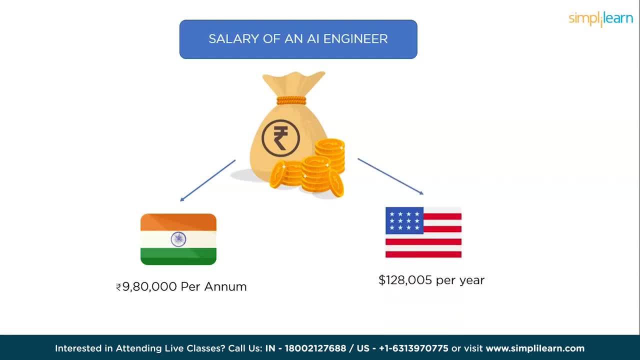 engineer in the United States is $128,500 per annum. It's worth noting that AI is a rapidly growing field in India, as there is a high demand for skilled professionals in this area, which can result in higher salaries and attractive compensation package for qualified candidates. 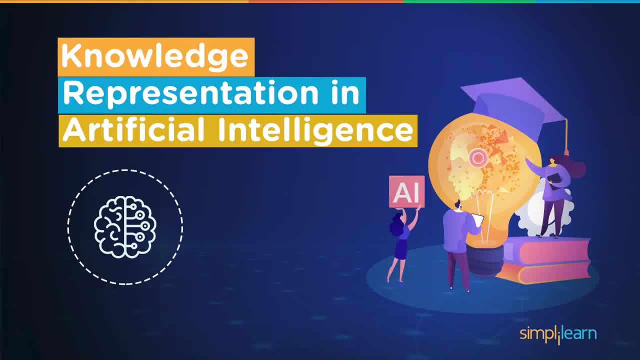 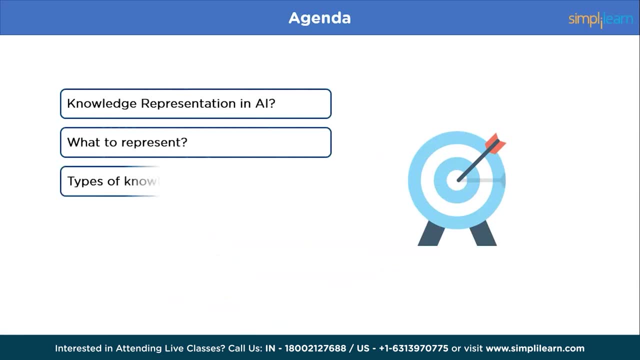 On that note, welcome to the Simply Learn YouTube channel. today we are here with an interesting video on knowledge representation in AI. Without any further delay, let's have a look at the agenda. So first we'll start with what is knowledge representation? next, what kind of knowledge? 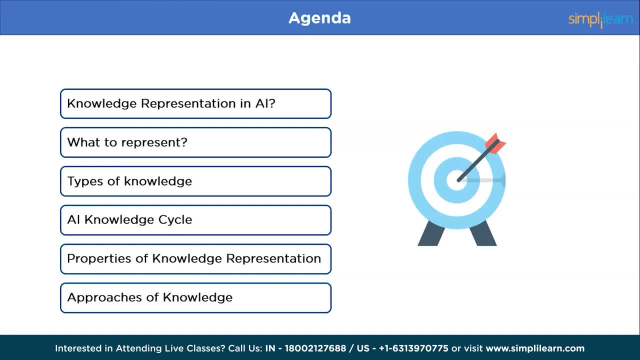 to represent. in AI advancing, we will understand the types of knowledge. moving ahead, let's have a look at the AI knowledge cycle and then the properties and finally, the approaches of knowledge representation. Before going deep into the topic, let us understand knowledge representation with an example. 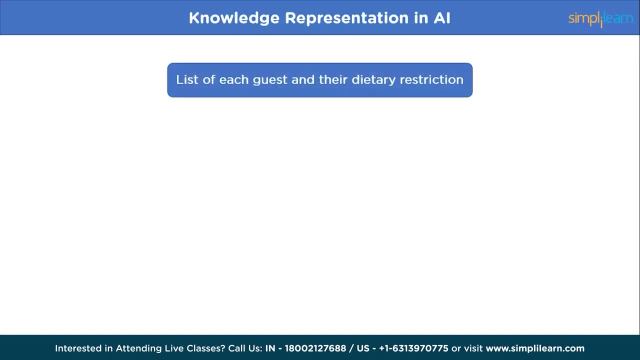 So, For example, if you are organizing a party and you need to keep a track of your guest's dietary restrictions, So you could represent this information in a table that lists each guest and their dietary restrictions. So in this table, each row represent a guest and the column represent their name and dietary. 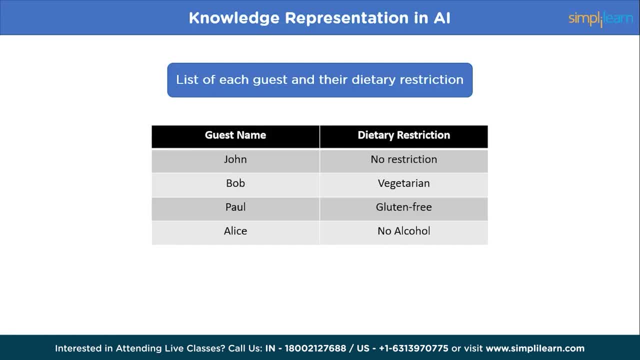 restriction. Organizing this information in a structured way allows you to reference it as needed throughout the party planning process quickly. So this is an example of knowledge representation, because you are using a system to represent information meaningfully that can be easily understood. It can be easily accessed and used. 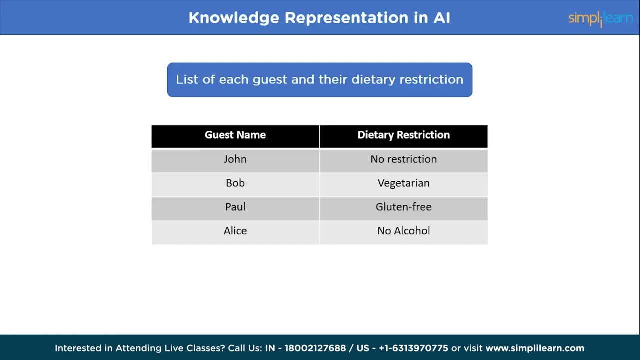 Other examples of knowledge representation include using a graph to represent relationships between concepts, or a decision tree to represent a decision making process. Now we got a basic idea of what is knowledge representation in AI. Moving ahead, let's have a look at the various kinds of knowledge that AI needs to represent. 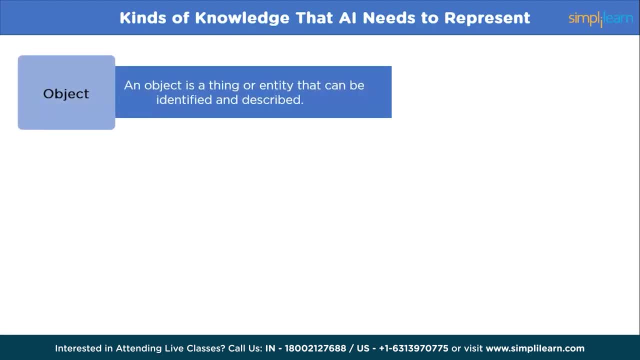 So first, Object. So an object is a thing or entity that can be identified and described. So, for example, a car, a person or a book. For example, there is a cold, There is an outdoor theater, There is a car. 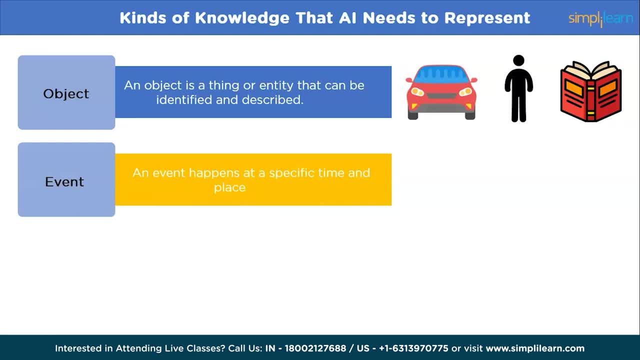 are all objects coming to events. an event happens at a specific time and place, for example, a wedding, a concert or a game are all events. next is performance. performance is a measure of how well a task is accomplished. for example, in sports, performance might be how many points a player. 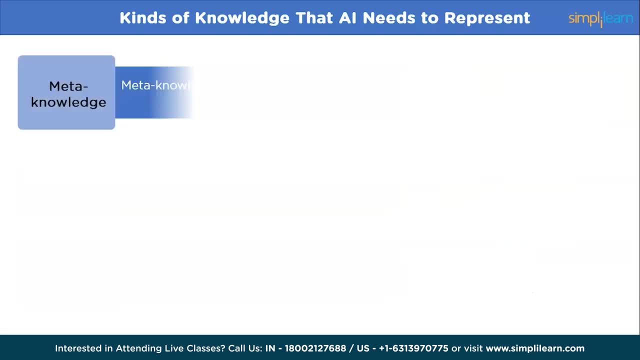 scores or how fast a runner completes a race. next we have meta knowledge. so meta knowledge refers to knowledge about knowledge. it is the knowledge that describes how other pieces of knowledge are related to each other. for example, knowing that a car is a type of vehicle is an example of meta. 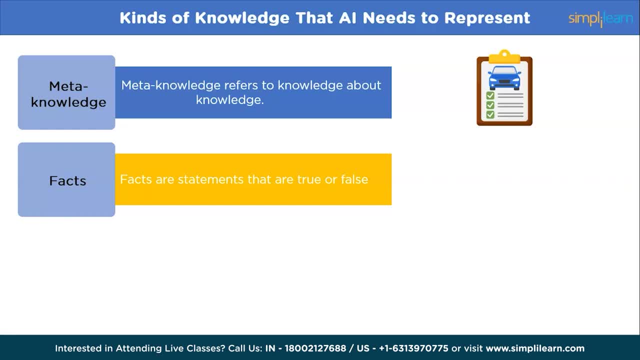 knowledge. next we have facts. so facts are statements that are true or false. for example, the sky is blue is a fact. knowledge base. a knowledge base is a collection of knowledge and information that is organized and stored in a specific way. for example, a customer information database is. 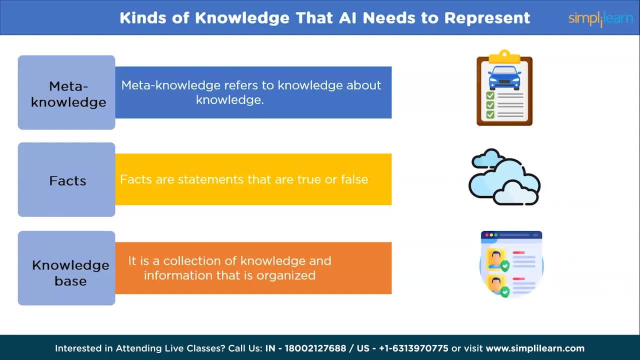 a type of knowledge base. the provider information database is a type of knowledge base. the provider. an example of these concepts: consider the domain of a car dealership. in this domain, an object might be a specific car model, such as the toyota camry, an event may be a test driver or a purchase of a car. 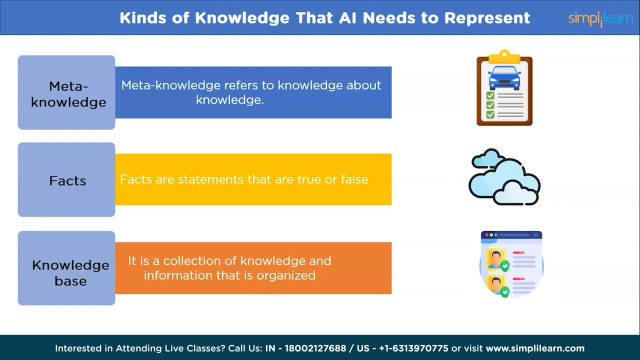 so performance might be how well a salesperson can sell a specific car model, and meta knowledge suggests that the toyota camry is a certain type. a fact might be that the camry has a particular fuel efficiency rating. finally, the knowledge base might include information about the customer. 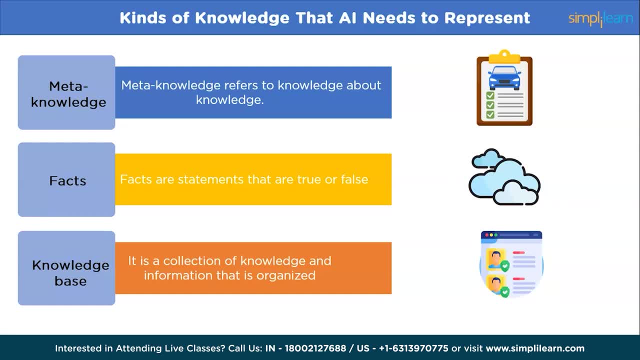 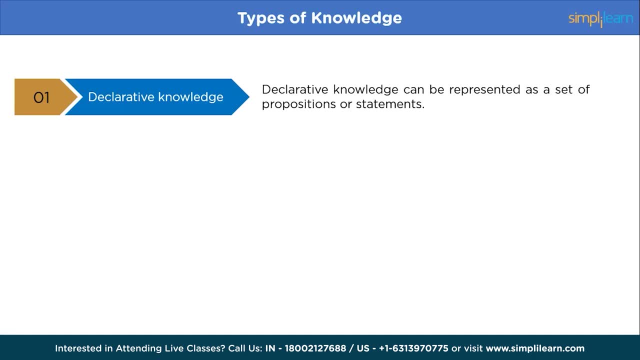 preference, sales data and vehicles specification. so next let's discuss on the types of knowledges. first we have declarative knowledge. this is factual knowledge about the world, including information about objects, concepts, events and relationships. declarative knowledge can be represented as a set of propositions or 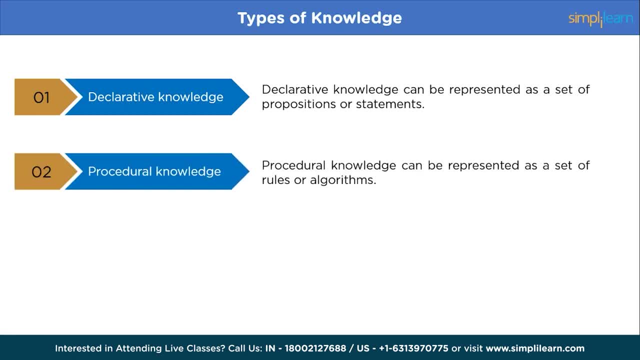 statements. next we have procedural knowledge. this is knowledge about how to do things, including skills, procedures and techniques. so procedural knowledge can be represented as a set of rules or algorithms. and next we have meta knowledge. so meta knowledge refers to the knowledge that describes or characterize other knowledge. it provides information about other knowledge properties. 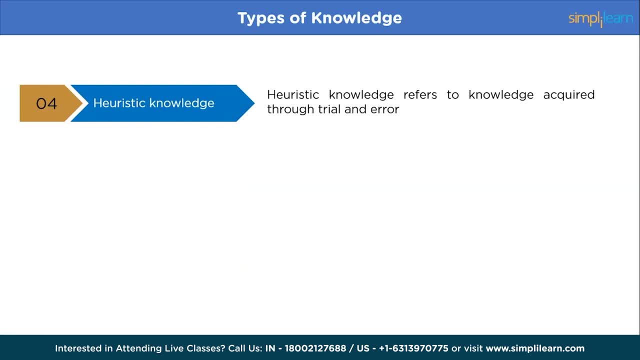 relationships and context. next, we have heuristic knowledge. refers to knowledge occurring those trial and error, and it often based on experience rather than formal rules or logical reasoning. and finally, we have structural knowledge. structural knowledge refers to the organization and arrangement of information or data meaningfully. structural knowledge is used to create model that describes the relationships between different. 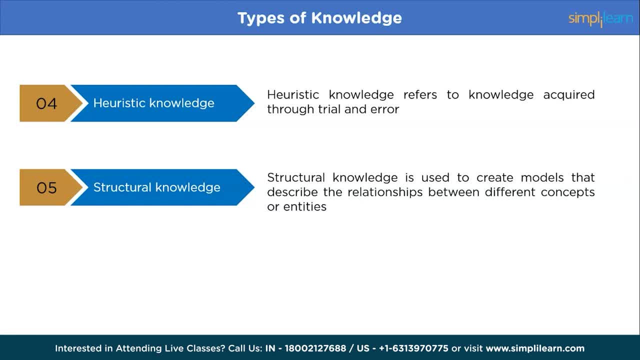 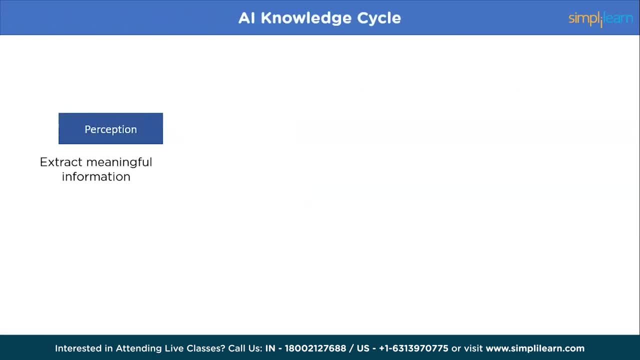 concepts or entities in knowledge representation. so, following to this, we have cycle of knowledge representation in ai. so perception. so perception is the process by which information is gathered through the sense and processed by the brain. in the context of knowledge representation, perception refers to the ability of an ai system to sense and interact with the real world and extract meaningful 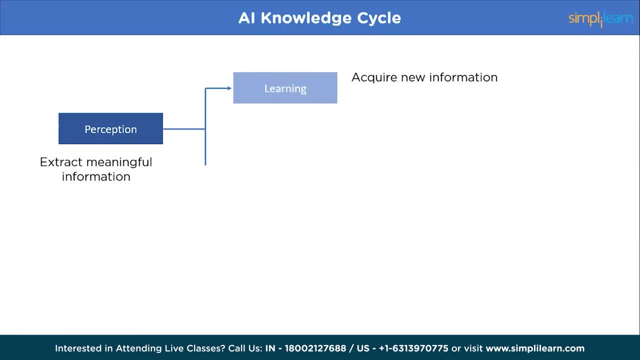 information from it. then we have this process of supercomputer. i'm also interested that the next- and Then we have learning. So learning is gaining new knowledge, skills or behavior through experience, study or instruction. In the context of knowledge representation, learning refers to the ability of a system. 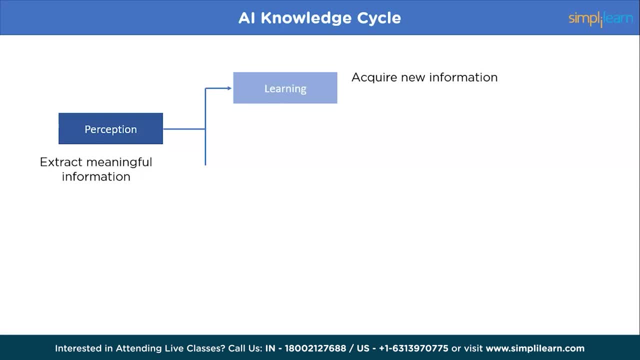 to acquire new information and modify its internal knowledge representation based on that information. And then we have knowledge representation and reasoning. So knowledge representation is creating a model of knowledge in a computer system that can be used for reasoning and decision making. The reasoning is used that model to conclude, make inferences and solve problems. 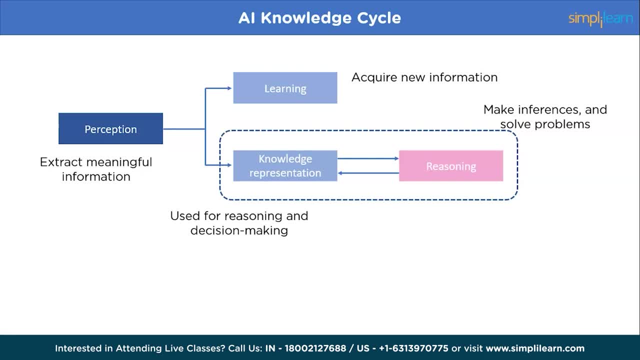 So, in the context of knowledge representation, the goal is to represent knowledge in a way that it is efficient and effective for reasoning. And then we have planning. Planning is creating a sequence of actions to achieve a goal. In the context of knowledge representation, planning refers to the ability of a system. 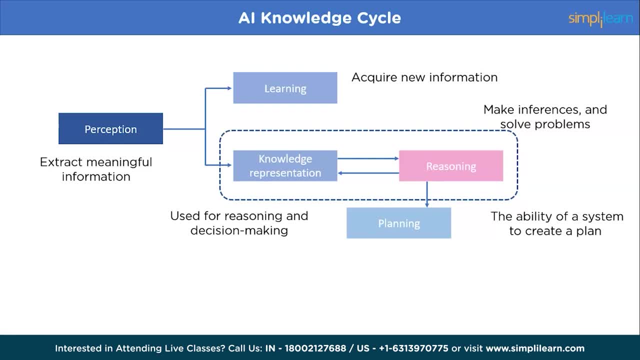 to create a plan of action based on its internal knowledge representation. And finally, we have execution. Execution is the process of carrying out a plan of action In the context of knowledge representation. execution refers to the ability of the system to implement a plan of action based on its internal knowledge representation and the 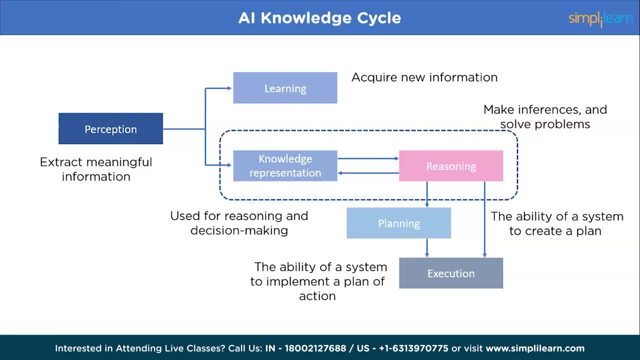 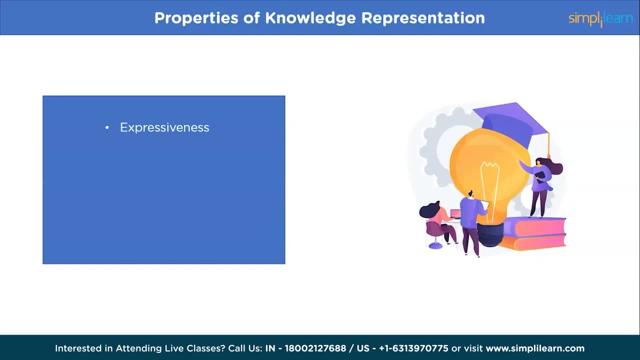 environment factor it pursues. Now let's discuss the properties- Three properties of knowledge representation, including expressiveness. A knowledge representation system should be able to express a wide range of concepts and relationships between them. The next property is inferential adequacy. A knowledge representation system should support the ability of a system to implement a plan. 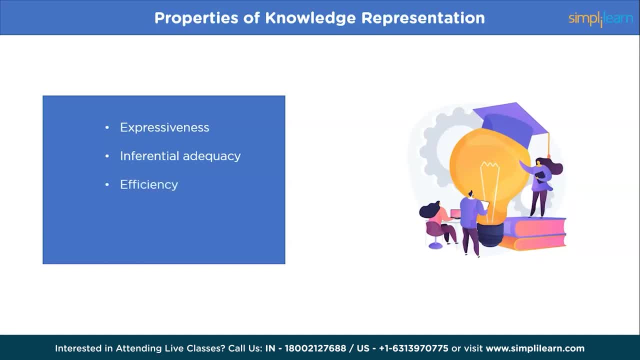 of action based on its internal knowledge representation. This means, in the context of knowledge representation, a system should be able to reason with the represented knowledge. The next property is efficiency. A knowledge representation system should be able to manipulate and retrieve knowledge efficiently. Next, 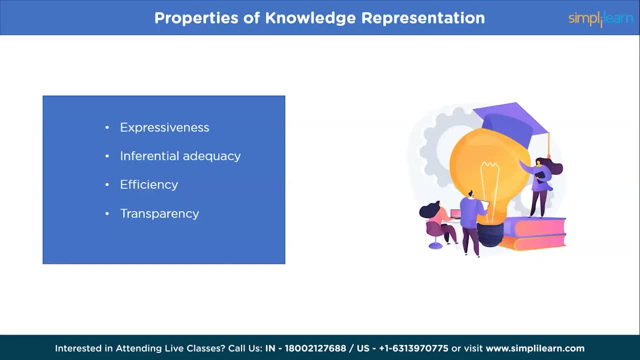 Transparency: A knowledge representation system should be transparent to the user, allowing them to understand and modify the knowledge quickly. And finally, scalability: A knowledge representation system should be able to handle large amounts of data and still maintain its efficiency and expressiveness, Moving ahead. 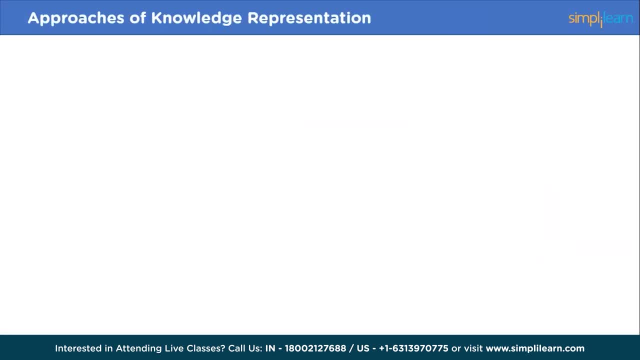 Let's have a look at the approaches of knowledge representation. Knowledge representation is an essential aspect of artificial intelligence. that involves organizing and structuring knowledge in a way that computer systems can effectively utilize. There are different approaches of knowledge representation in AI, including simple relational. 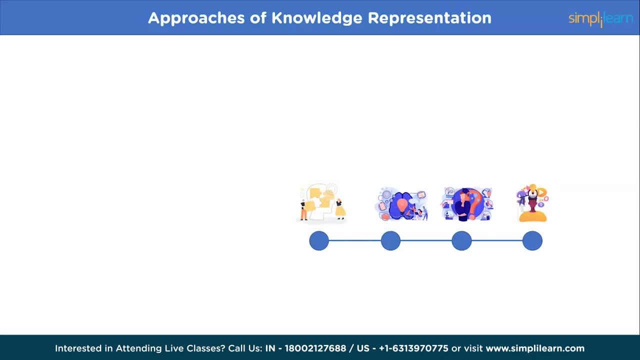 inheritable, inferential and procedural knowledge. So let's explore each of these approaches of knowledge representation with an example. First we have simple relational knowledge. This type of knowledge representation involves organizing knowledge through relationships between entities or objects. Simple relational knowledge is typically a set of rules defining the relationships between 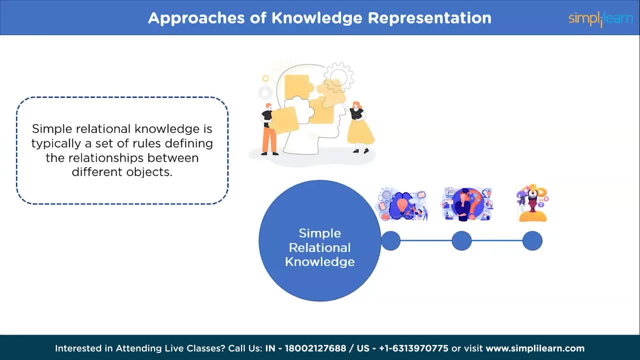 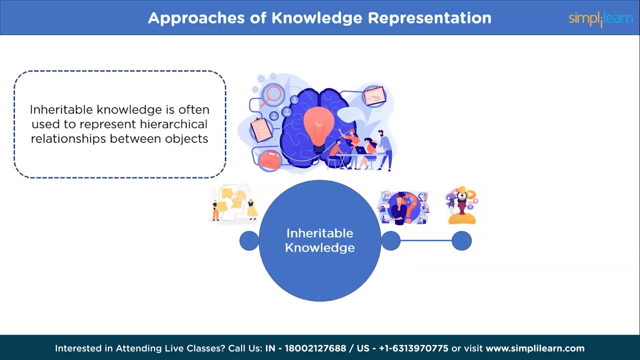 different objects. For example, a simple relational knowledge representation for a family could be: John is the father of Mary. Mary is the sister of Peter. Peter is the son of John. Next, inheritable knowledge. Inheritable knowledge represents the knowledge that can be passed on from one object or entity. 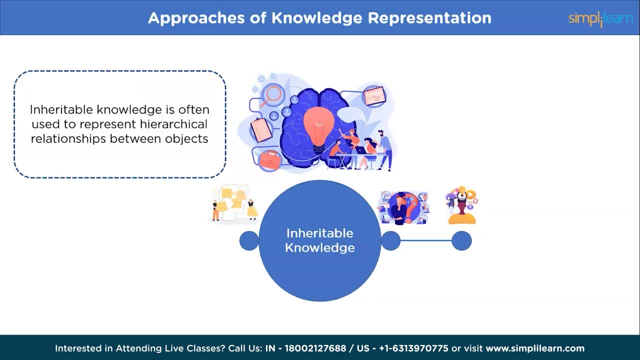 to another, So this type of knowledge representation is often used to represent hierarchical relationships between objects. For example, an animal that belongs to the class of mammals inherits all the attributes of its parent class, So in this case the inheritable knowledge is represented as mammals are warm-bladed. 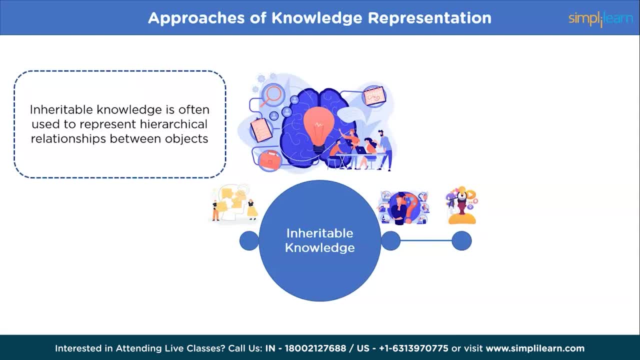 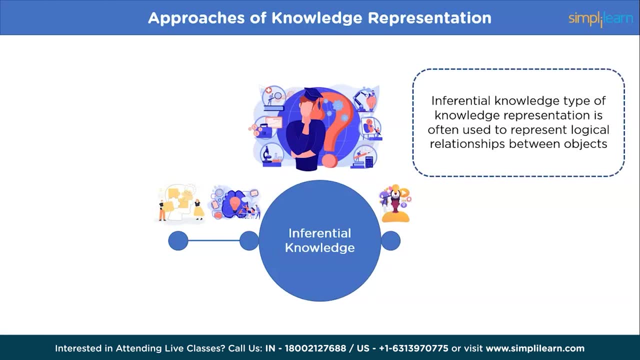 animals. dogs are mammals, therefore dogs are also warm-bladed animals. Next, inferential knowledge. Inferential knowledge represents knowledge derived from another knowledge, So this type of knowledge representation is often used to represent logical relationships between objects. For example, in a medical diagnosis system, a doctor might infer a patient's condition.